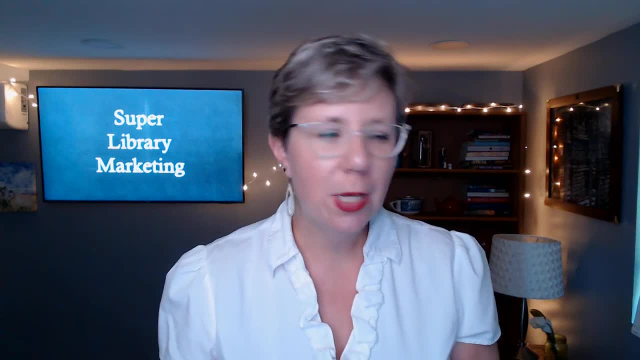 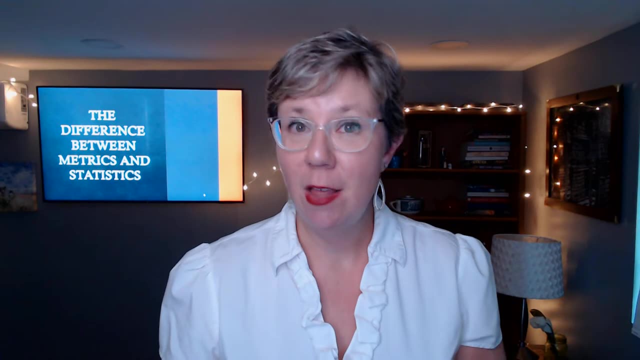 important because there are two terms that we sort of use interchangeably when we talk about marketing And I want to make sure we know the difference between metrics and statistics. They both have a place in our work, in promotions. So here is the definition, So we can talk about them. 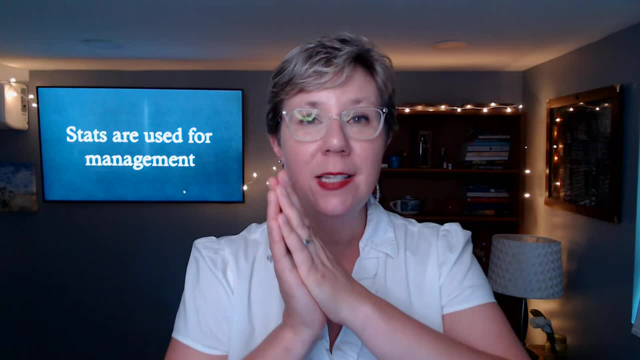 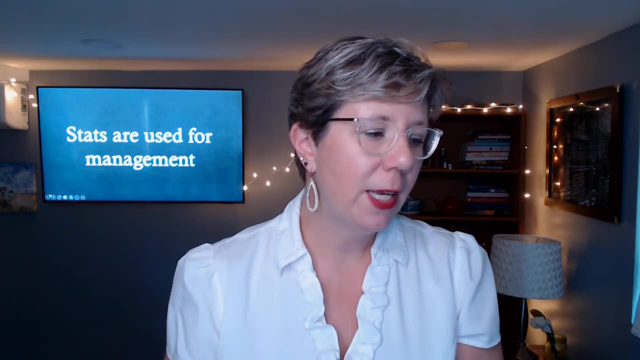 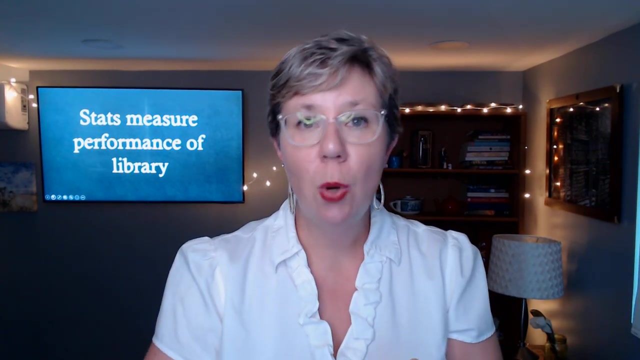 and talk about them in a way that's going to help us. So statistics are used for management: management of your library, management of your department. They include things like your total circulation, the number of people who visit your library on any given day, the total overall use of your database. 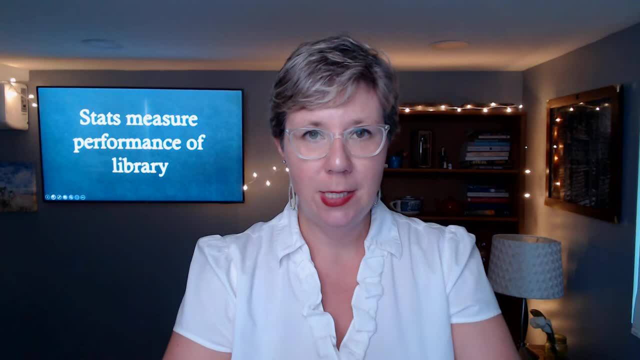 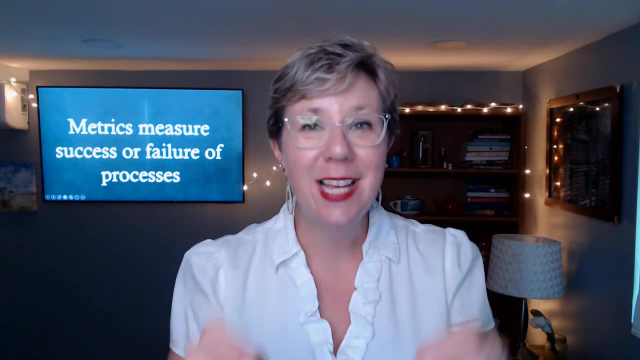 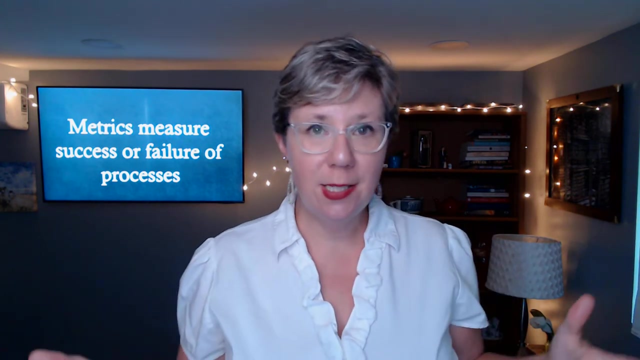 These things measure the performance of your library statistics. That is different from metrics in that metrics measure the success or failure of processes. So let's take total circulation. total circulation is a statistic for your library. Now, when you take your total step circulation stat. 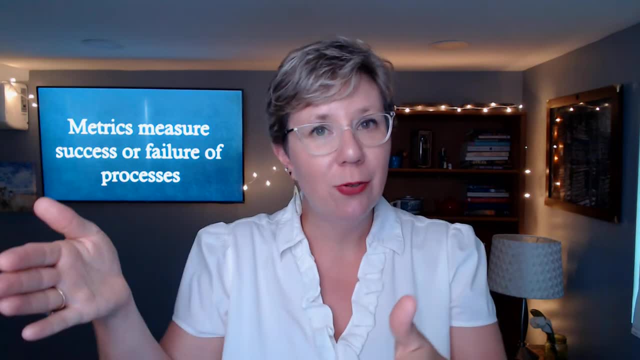 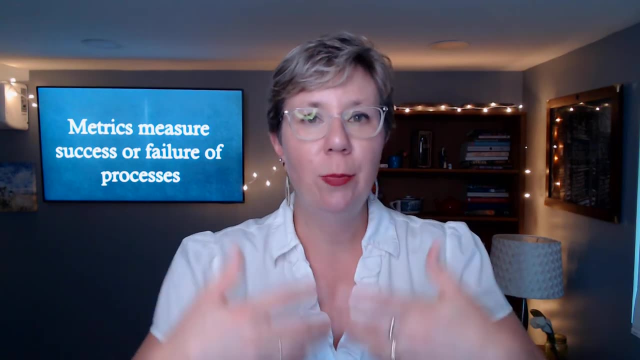 and you compare it with the year before and you see an increase or decrease. that percentage is a metric because that tells you whether your promotions and your processes are succeeding or failing. It's very squishy the line between the two, but it's super important. 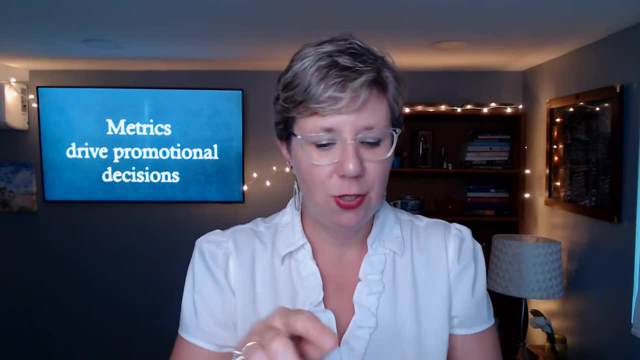 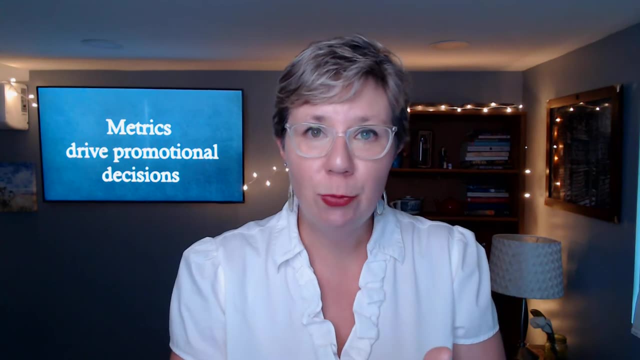 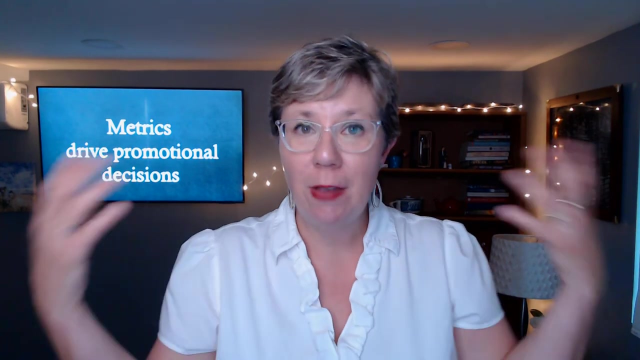 Metrics drive your promotional decisions. So for marketing, that includes things like your click rate, your open rate, to some extent the engagement rate of your social media posts, your net promoter score, which is how people feel about your library, whether they view it. 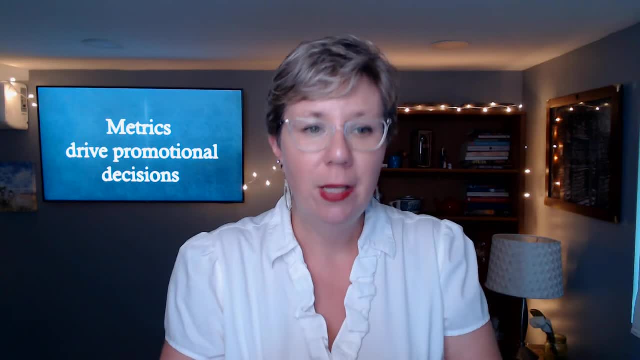 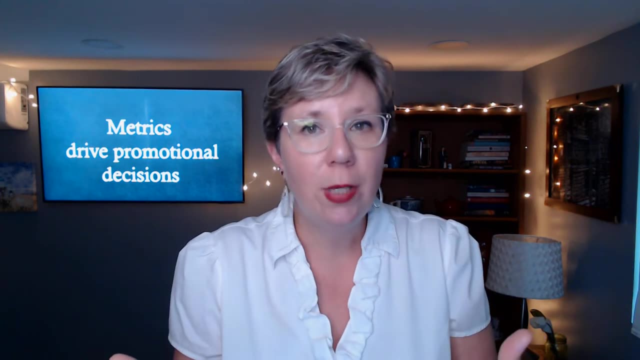 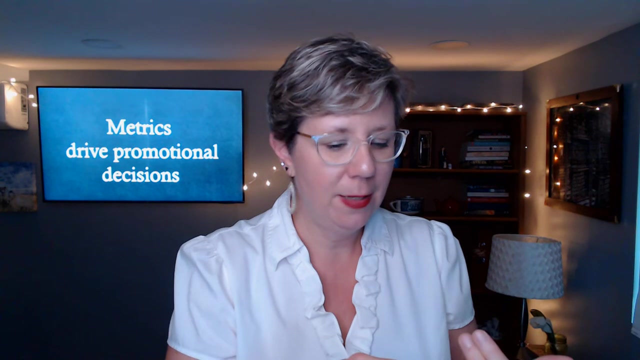 in a positive light if that goes up or down. that is a metric. Knowing those metrics drives your promotional decisions. Statistics are just showing you how your, your libraries, performing, but metrics can tell you what is working promotional wise, so you can repeat those things, And it can. 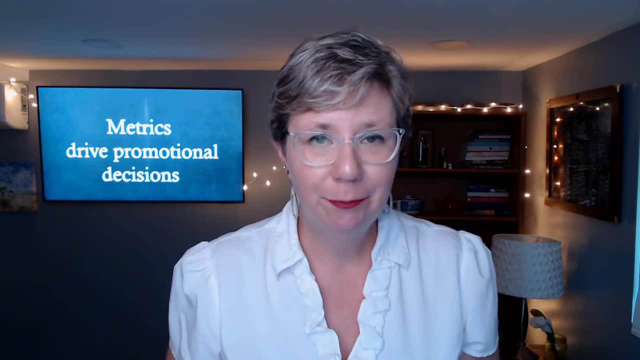 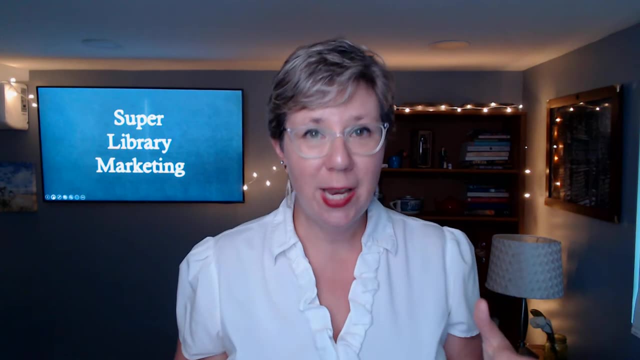 tell you what is not working So you can delete the things that aren't working. So I hope those two definitions have helped you. We sort of use them interchangeably. I'd like us not to do that anymore. I'm sure you have comments or questions. How do you use statistics and metrics in your own? 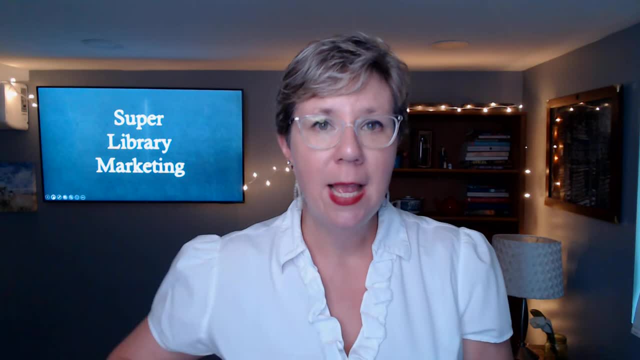 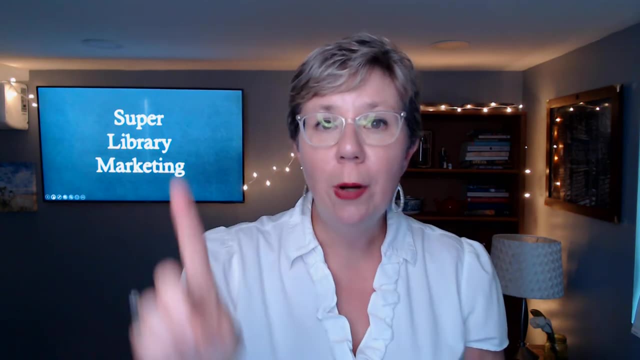 library promotions? I would love to know. Let me know down in the comments. Head to superlibrarymarketingcom. Click on the library marketing show tab to suggest a topic for a future episode or to nominate your library or another library marketing show. If you have questions.